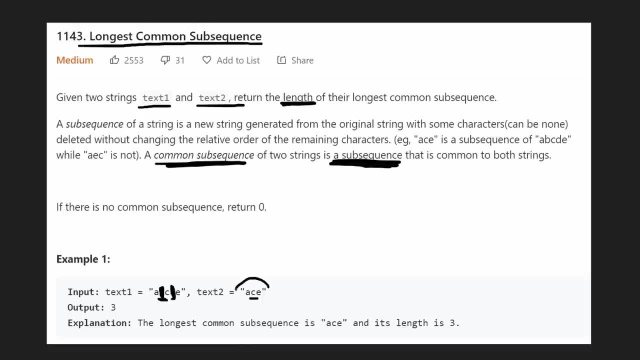 So we get the longest common subsequence to just be the original second string, right ace, because ace can be found in the first string. All we have to do is remove a couple characters right, Remove the b and remove the d. then we get a subsequence that matches the second string. 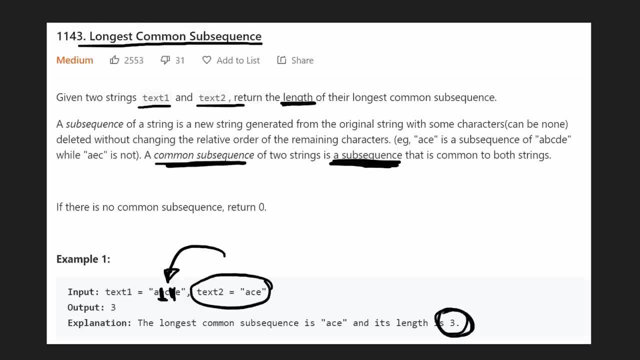 So the length of the longest common subsequence is three. So how can we solve this problem? Well, as I mentioned, dynamic programming is the most efficient way to solve this problem. But before we even get into the dynamic programming solution, which is going to be a two-dimensional dynamic programming, 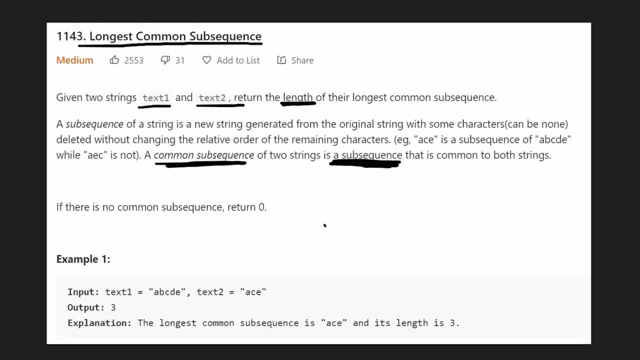 solution. before we get into that, let's just notice one thing. Do you so? let's say, these are our two strings, right, String one and string two. Does it at least make sense to you that? okay, like we would want to start, let's say at the beginning of both strings. right, Like we're? 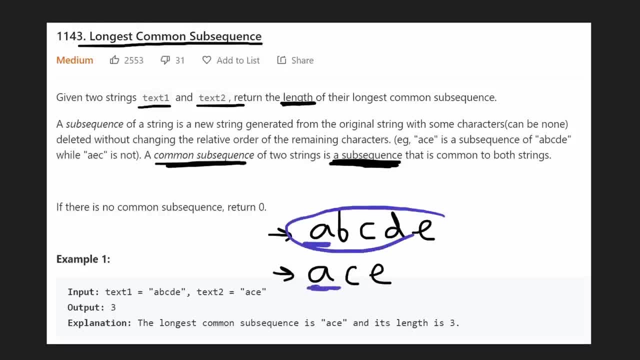 looking for the longest common subsequence. It might just be that both of the strings are actually equal, right? That could be a possible way. So let's look at the first character in each string, And in this case they match each other, right? They're the same character, So does it at least? 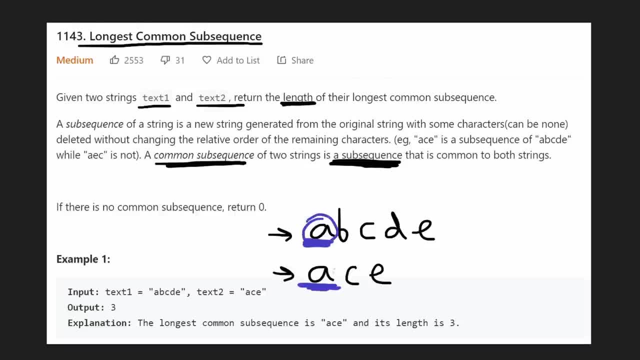 make sense to you that if both of the characters match each other right- The first characters, that the longest common subsequence- then we can break it into a sub problem. right Now. the new problem we're looking at is finding the longest common. 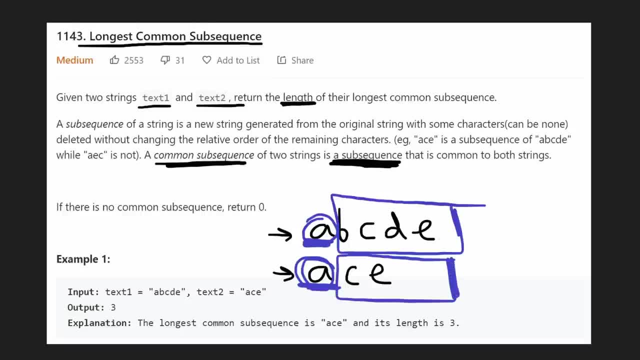 subsequence between the remainder of both strings: right Plus one plus one. because we see that the first two characters are equal. right, That's where our one comes from. right, Because we know that the longest common subsequence is at least going to be one. because we found a matching pair. 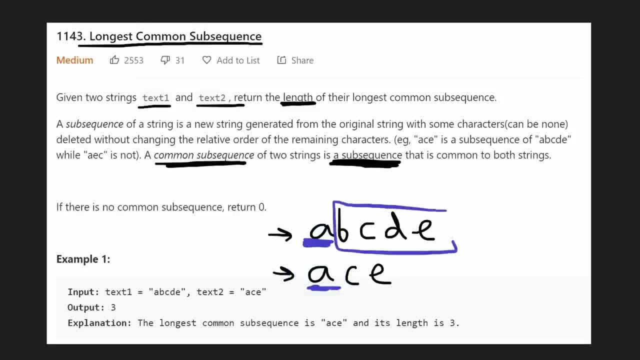 of characters, right, And then we have a sub problem, Right, And you might know that that's what dynamic programming is all about: finding the sub problem. Now, what if this character was a B, right, And this is an A? So clearly they're not. 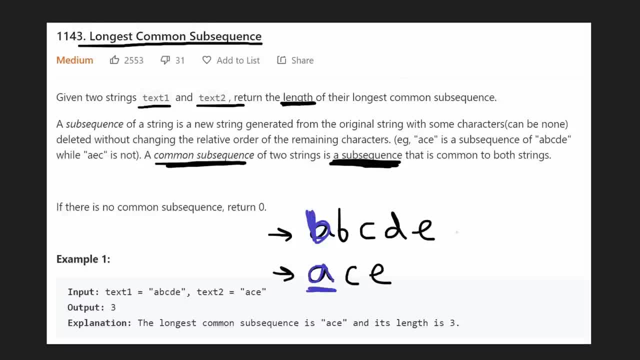 the same character. What would we do then? Well, we can't do what we just did. We can't add one and then find the longest common subsequence between the remainder of the two strings. We can't do that, but we can break it into a. 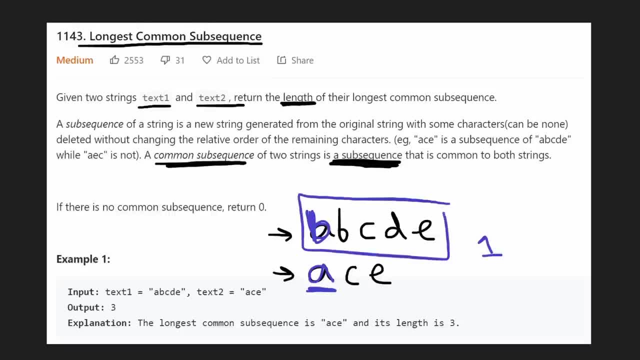 sub problem. We can say: well, it's possible that the longest common subsequence could be between these two strings, right? Or it could be between this string and this string. So this is just a little bit of an explanation before I show you the actual dynamic programming solution, right. 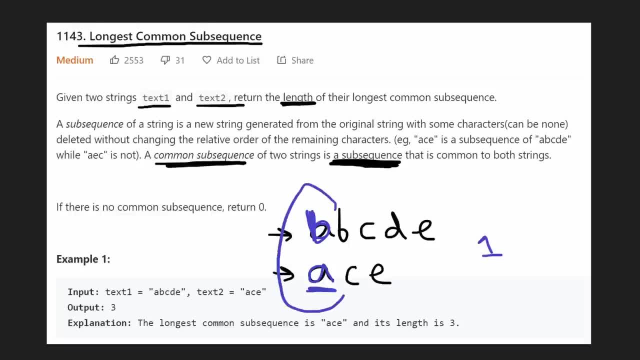 Basically, what we found out is that, based on comparing the first two characters, whether they're equal or not equal, we can break up the problem into sub problems and then solve the problem. So we can say: well, it's possible that the longest common subsequence 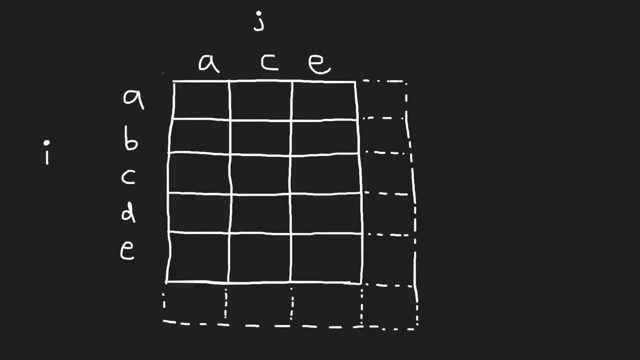 could be between this string and this string. So this is just a little bit of an explanation before we solve those sub problems. So take a look what I just did: I took the two input strings right- String one and string two- and I wrote them in a different way. right, I said that this. 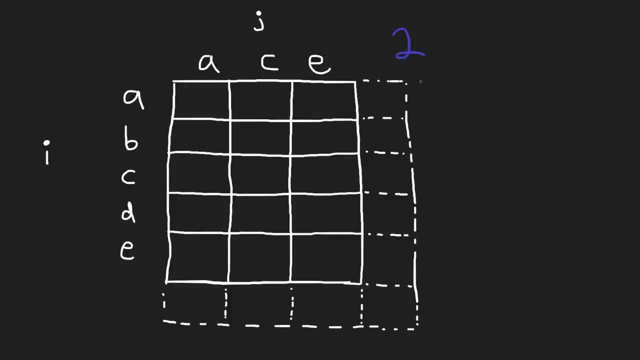 is a two-dimensional dynamic programming problem And you might know that a grid, a 2D grid like this is commonly used to solve these types of dynamic programming problems. So notice that for each character in both strings there's a square right A position a. 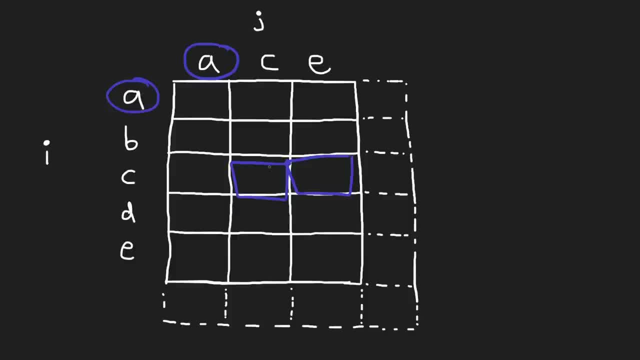 cell that we can put a value in. we're going to put a value in each of these cells, and so let's just start at the beginning, like we did, right? so let's start at the first characters, right? what we're trying to do is for these strings find the longest common subsequence between the entire strings. 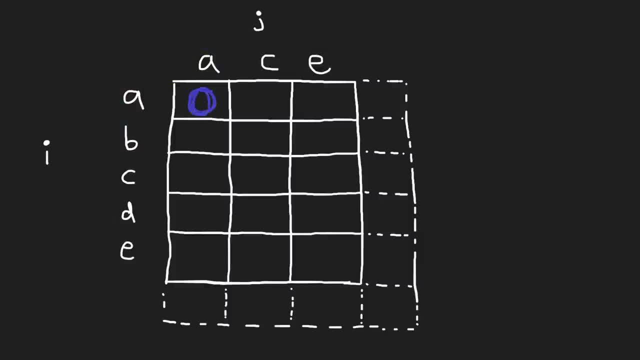 right. so what we're going to do is put that value right here. that's what's going to be the entire longest common subsequence. so we want to compute the value that goes here, but what you're going to find is to do that we need to solve some sub problems and then you know, continue to do that. 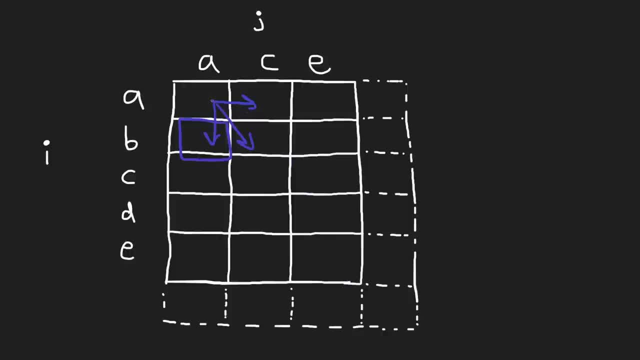 and then work our way back up to this position. so what do we notice? we let's look at these two characters. right, they're equal a and a right, so okay. so now we want to find the value that goes here. how can we find that value? well, like i mentioned right now, 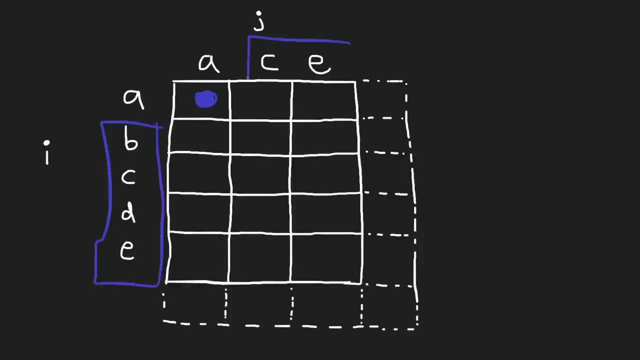 we're trying to solve a sub problem. We want to find the longest common subsequence between these two substrings- right? We don't have to check these A's anymore because we know they match each other. So now I want to find this new sub problem right, And so basically what I'm saying. 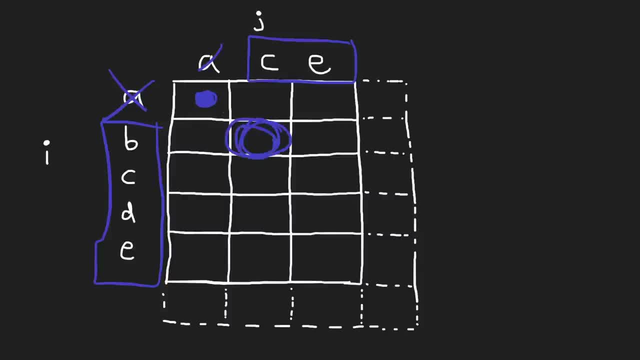 is. I'm going to go here. I want to solve the sub problem that goes here. So now we're here. we're comparing this B with this C. We see that they're not equal. this time, right. That means we're not going to be going diagonally, We're not going to look at this sub problem, We're going to. 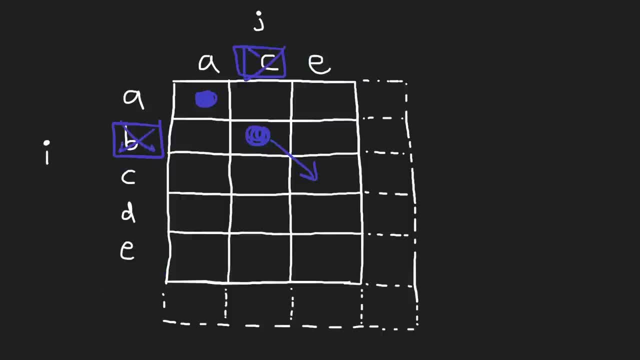 look at a different sub problem. Since these characters do not equal each other, we have to check two different sub problems. It means that the longest common subsequence between these two substrings is going to be found in either of these two positions, right? So let's look at this. 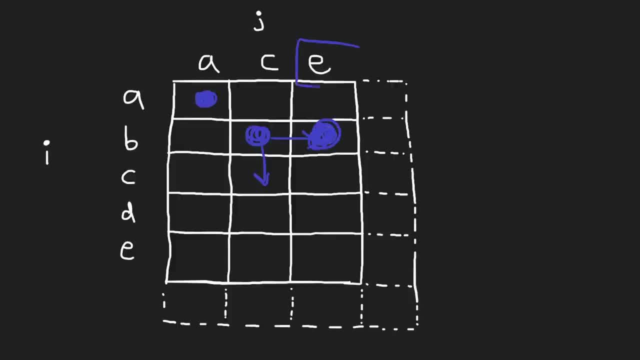 position. first, What this position tells us. we're trying to find the longest common subsequence between this string and this string, And so what we're going to do is we're going to look at this string and this string, right? So basically, we're not looking at this C anymore, right? And this? 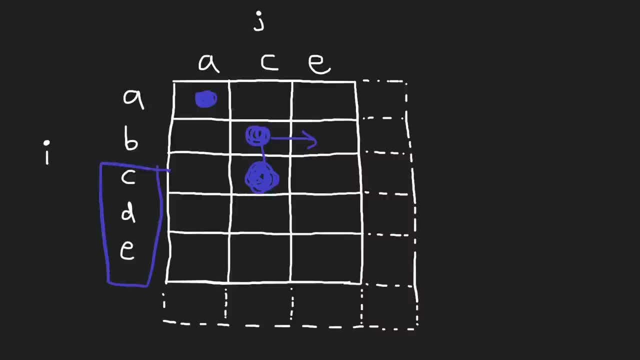 position tells us that we're looking at the longest common subsequence between this string and this string. So basically, when we remove this B right And just by looking at it right, you can tell that this is going to: these two strings are going to lead to a longest common. 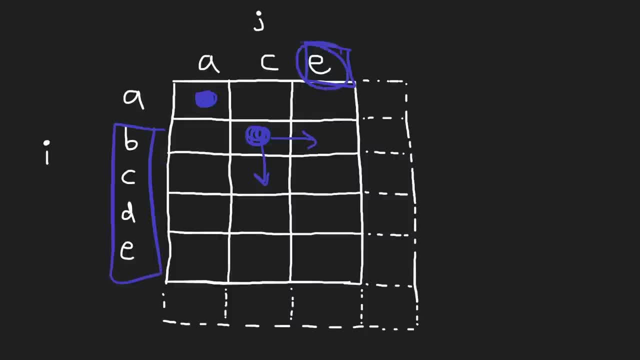 subsequence of one. Just by looking at it right, Because you can see that this has one character: it's an E. it only matches this E, so that's going to be a one. But when you look at this string and this string right corresponding to this position, we see that this has a CE. 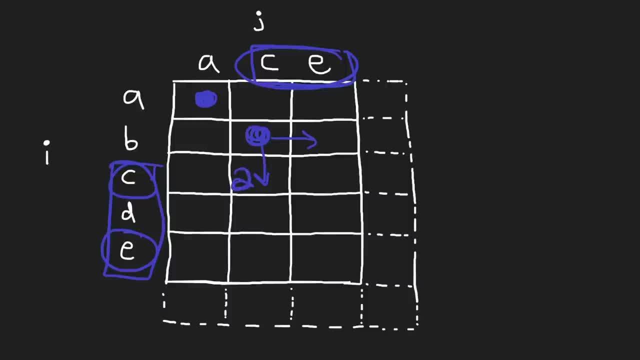 this has a CE, so this is going to end up being a two, But let me actually solve the rest of it a little bit. So, mainly looking at these two strings right in this position, we see that the C's match each other, right. So since remember when the characters match each other, 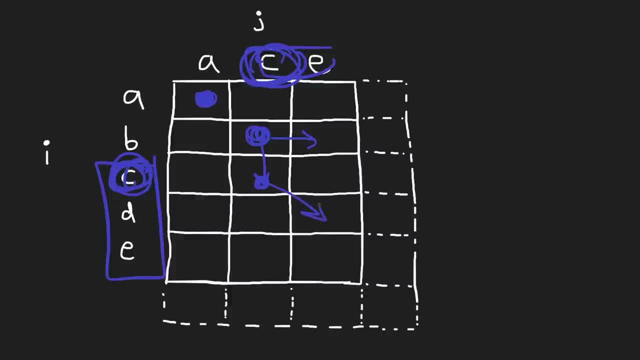 the first characters of both strings match each other, right? So, since remember, when the strings match each other, that's when we go diagonally, And the reason we go diagonally is because then we know we can look at the remainder of both of the strings, right, We know that this. 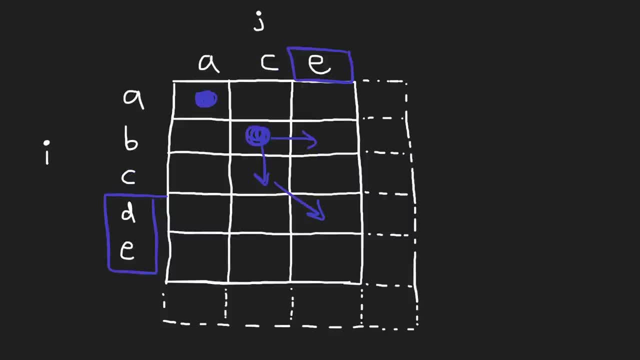 C matches this C. so we want to look diagonally, We want to look at these two substrings. So what's the longest common substring between these two? Okay, so what are we going to do? Let's compare the first character, right? So D and E. So these characters are not equal. So remember what we do. 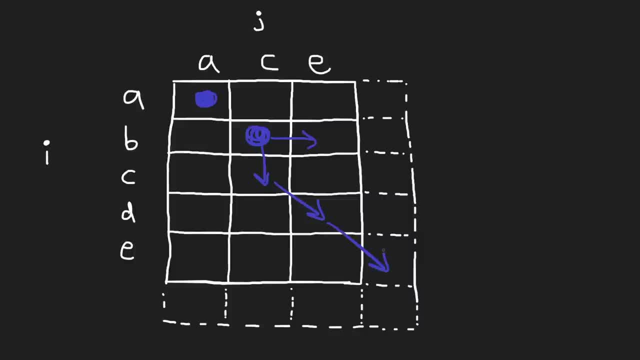 when the first character is equal. So we're going to look at the remainder of both of the strings, right, So these characters are not equal. Then we can't go diagonally. So what do we decide to do? We go to the right and we go down and we take whatever the max of these two is and then put it. 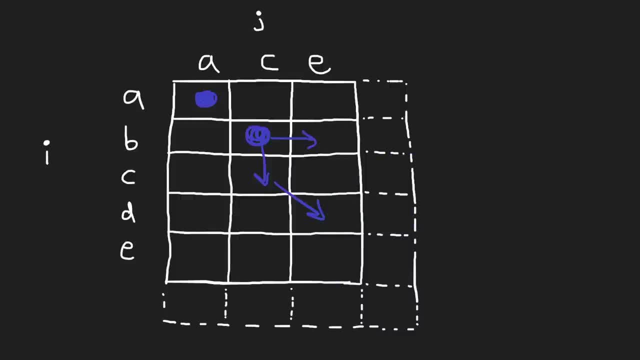 in this value. That's what we're going to do, So first let's check this right position. So what does this right position even mean? It means we're taking this substring and finding the longest common substring with this substring, but this is an empty string. So what's going to be in this? 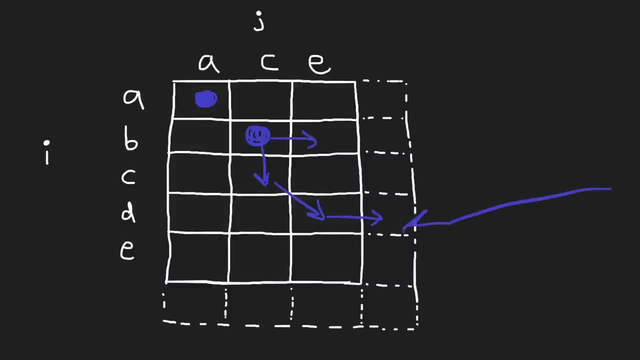 cell. Remember, we're going to look at the remainder of both of these strings, right? So remember, this is actually out of bounds anyway, right? So what default value are we going to give ourselves if we go out of bounds? to the right? Clearly, the longest common substring between a. 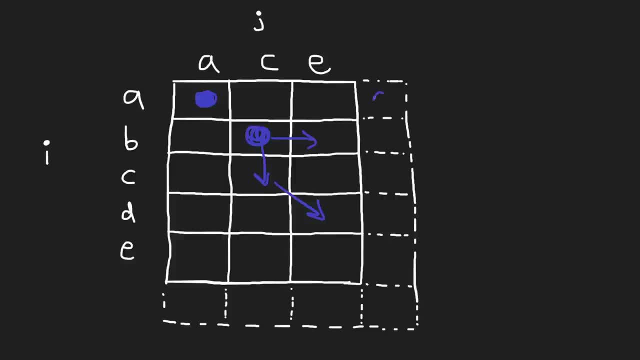 string and an empty string like this is going to be zero, right? So really, what we're going to initialize is we're going to say every value in this column is going to be zero. Similarly, this is an empty substring. If we were trying to find the LCS, the longest common substring between this: 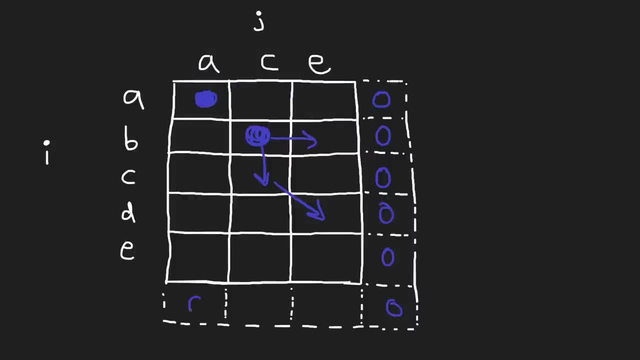 and an empty substring, we're going to say that this is an empty substring, So we're going to initialize our 2D matrix when we start the problem. Okay, so remember what we were doing. we were at this position. we were going right and we were going down trying to find the maximum. 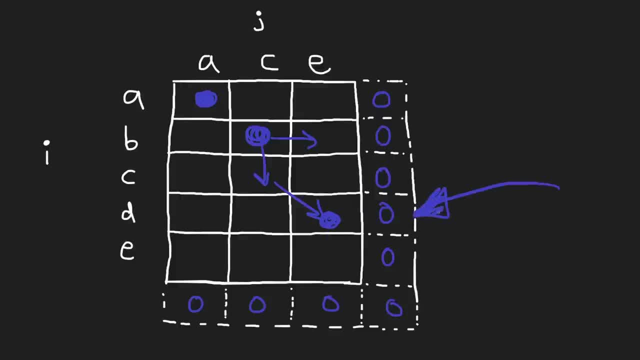 value. Well, clearly, to the right, we get a zero. So that's not the max, So let's go down. Okay, now we're down. So what are we doing? We're finding the LCS between this substring and this substring. Well, they're the exact same: right E matches. 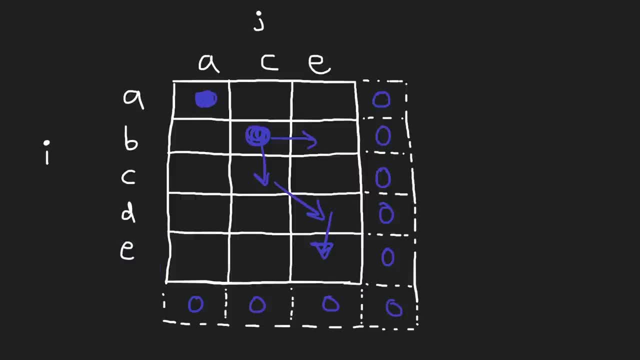 E, Okay, great. And remember when characters match each other, that's when we look diagonally right. So we came down here and now we're looking diagonally clearly we get a zero here, right? So zero plus one. the reason we're doing a plus one here is because we found 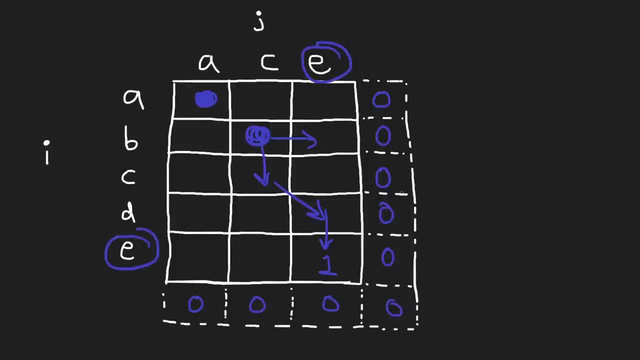 matching characters. When characters match, we add one because clearly the LCS between these is going to at least be one right- At least one of these characters matches. So now I'm basically going to go here and then take us back along the path that we came from and then show you what the 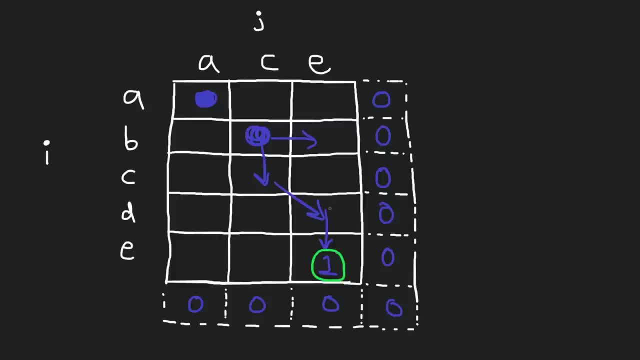 solution is: So we had a one here, right, And so from this position, we went down. So, since we were going down, that means that this character and this character did not match each other. So what we're going to do is just take the one and put it up here, right? So there's going to be a one here. 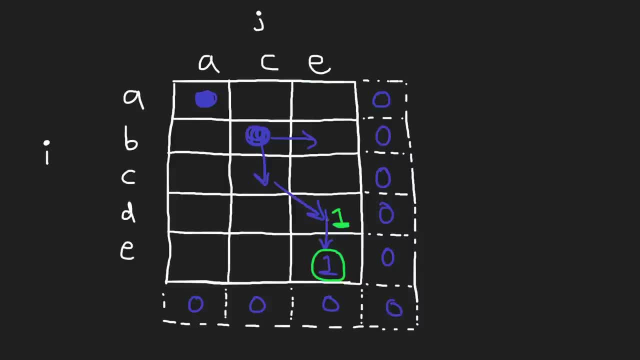 because the LCS between these two is one. But now we're going to go back over here diagonally, right? So diagonally means that this character matched this character, right? So we're going to take the value that we got up here, put it over here and add one because, remember, these match each. 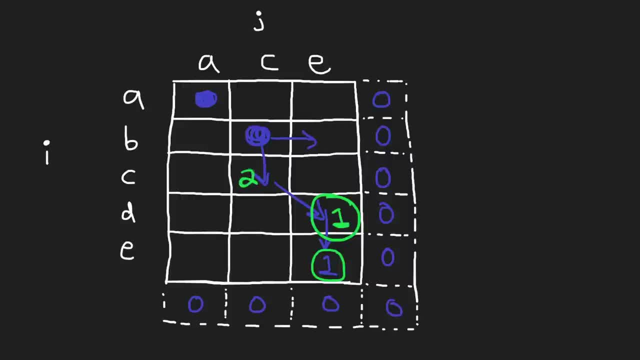 other, So we're adding one. that means we're going to end up putting a two in this position. And now we're going up. right, We're going up because that's where we came from, And remember, when you go up, that means the characters did not match each other. the C and the B don't match. 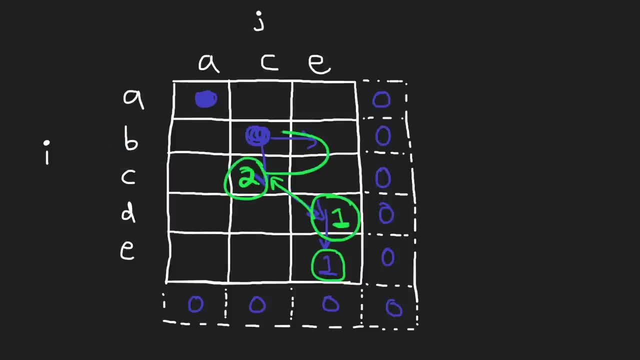 each other. So we're going to put a two here, right? We're just taking this two and putting it over here And, lastly, we're going back here. That's where we came from, right, Diagonally That. 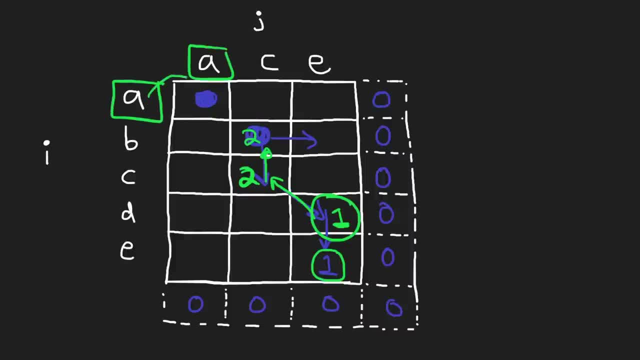 means the characters were matching each other. So we can add at least one character. So two plus one, that's going to be three. This is how we got the result right. So we got a three, meaning that the LCS between these two strings is three. right, And that's what we learned from the problem. 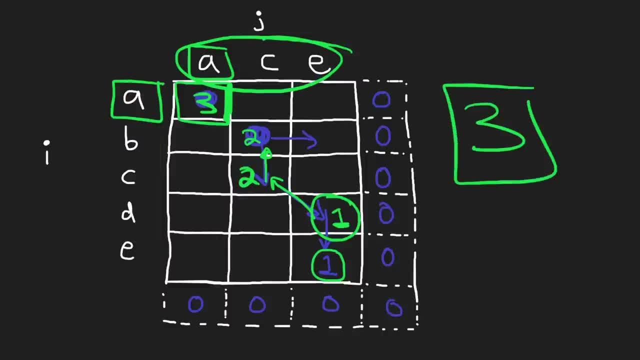 explanation. So right, what we're going to do is return three. that's our result, But you can see that the way I did it was basically intuitive, right? I used this picture and basically solved this problem by hand, using a little intuition and 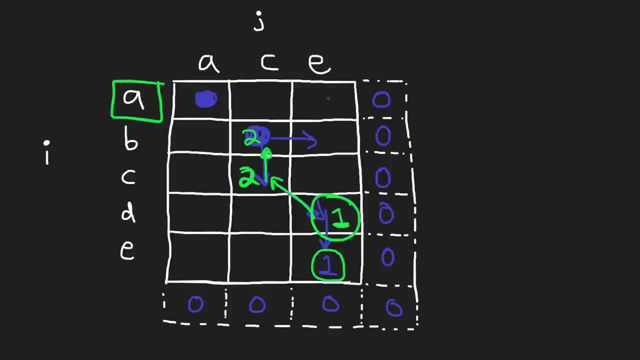 stuff, right. But the way we're going to have to solve this with code is going to be brute force, ish- right, So it's dynamic programming. But what we're going to have to do is for every value in this cell, right, So we are going to initialize these zeros- right, But with this matrix- right. 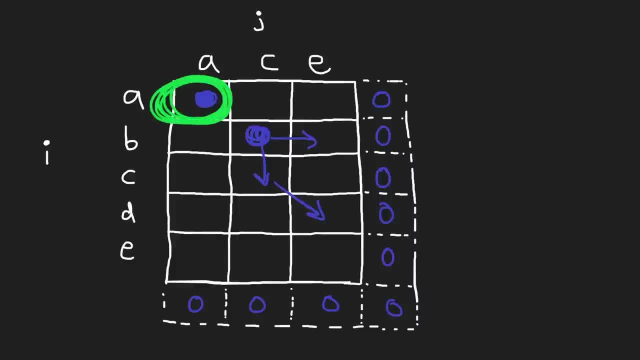 this 2D matrix. we want the value that goes up here, right, And to do that, we have to compute the value that goes here, that goes here, that goes here And basically for all these, and then finally we'll be able to have the value that goes here, which is the result that we're going to. 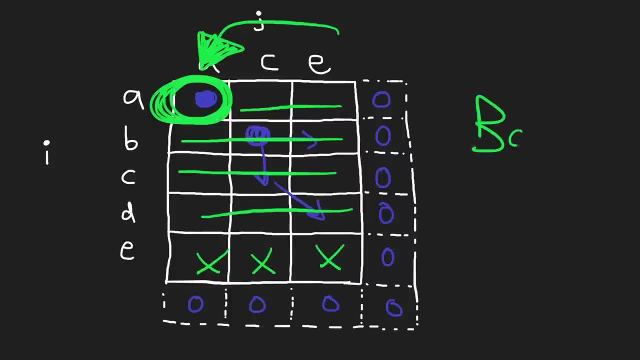 return. And so, basically, what I'm saying is this is going to be a bottom up dynamic programming solution, right Bottom up, meaning we're going to solve it in reverse order. we're going to first get every value, we're going to get the value that goes here and then work our way up until we get. 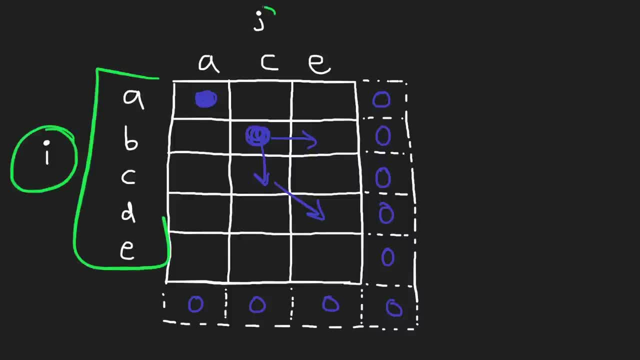 to the bottom. So what I'm going to do is we're going to do this right. So we're going to look at the column. I have a J that tells us actually the column and the I tells us what the row is. 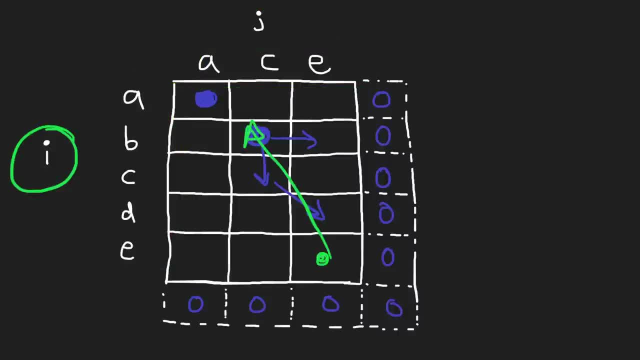 And so when we're working our way, starting at the bottom and working our way up, how are we going to determine what value goes in each cell? Basically what I went over earlier, right? So we're going to look at the characters And if they match each other, what we're going to do is say one plus. 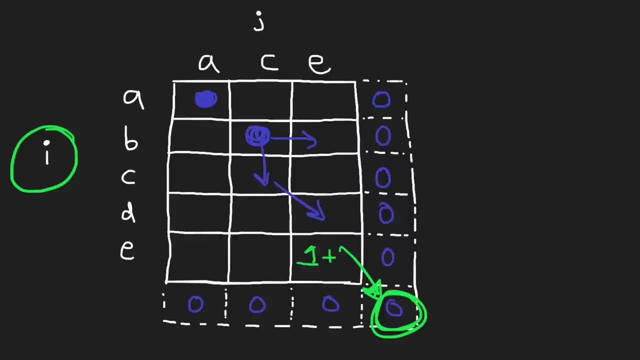 the value. that's diagonal right And we know when we go out of bounds there's a zero right, There's an imbalance right. So we're going to look at the values that go in each cell right And we're 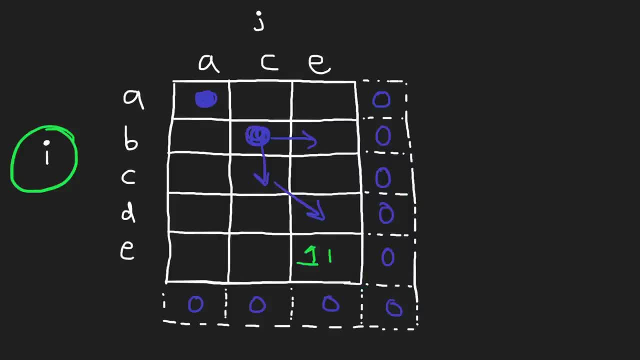 going to do that with every single cell, right? So when you look at these two, we get an E and a C, right, And when characters don't match each other, right. That's important. What we're going to do is we're going to look down, right, We see a zero down here, and we're going to go right, right to 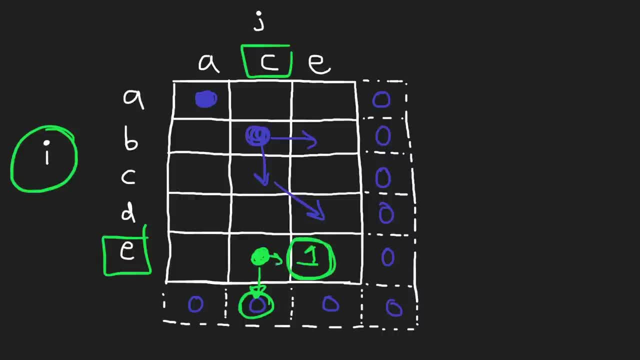 the right side And we see a one here on the right side, And what we're going to do is take the max of those two values And we see that the max is, of course, one right. One is bigger than zero, And 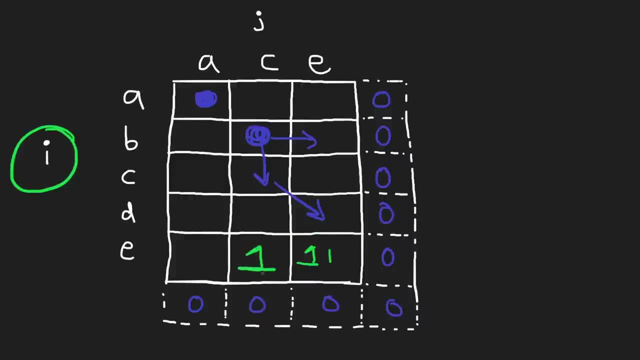 then we're going to do that with every single cell, right? So when you look at these two, we get an E and we're going to put that max value in the cell. So that's really it. There are two choices, right? 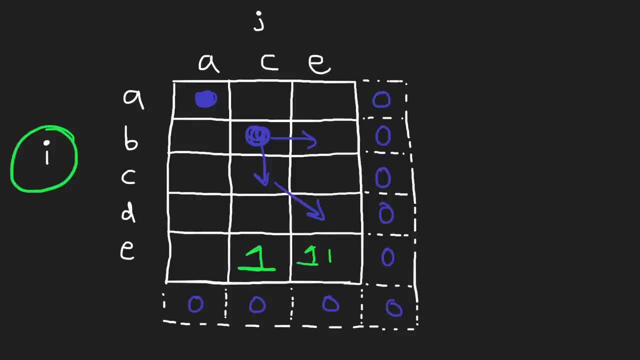 If the characters don't match each other- right in this case. or if the characters do match each other- in this case, right. That's basically how we're going to solve this problem. It'll make a little more sense when I show you the code. So, remember, we're going to have a 2d grid, So I'm 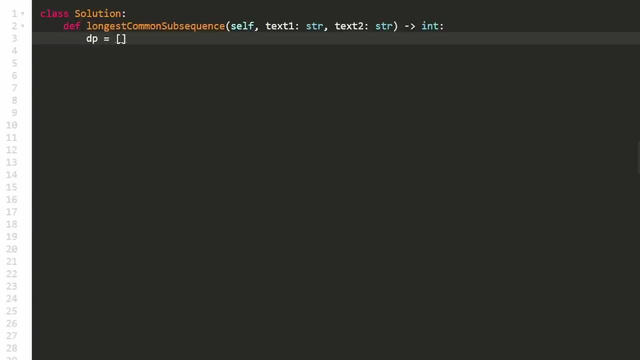 going to call that DP for dynamic programming. it's going to be a 2d grid And what I'm initially going to do is set it to all zeros, right? So, and I'm just going to do a little bit of Python stuff, So list comprehension in Python. So we're going to go through every single value. 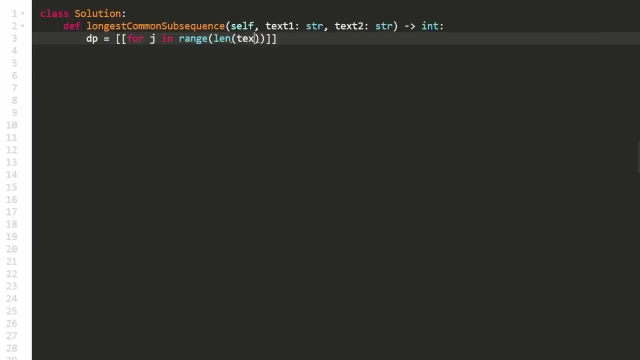 in the length of text, two plus one, right plus one, because we know that we need at least one more column to have all the zeros in it, And so we're remember we're going to put a zero for every value in that. So length plus one, and we're going to have this row for every value. 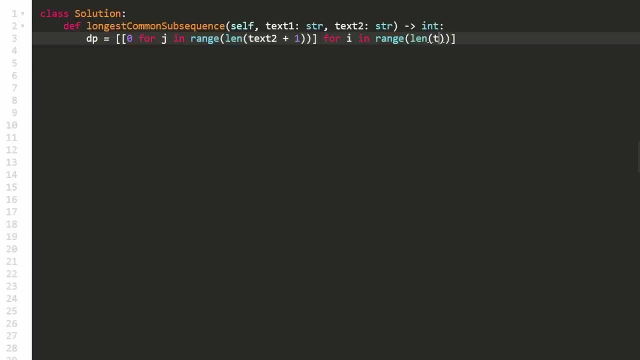 in that. So we're going to put a zero for every value in that, So length plus one. and we're going to put a zero in the length of string one, so text one plus one as well, right? So we're basically. if you're not familiar with Python, this looks complicated, But basically we're. 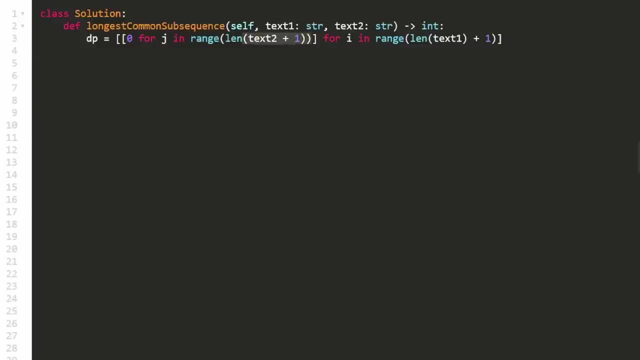 getting a 2d grid of dimensions length two plus one times length string one plus one, and initializing it to all zeros, And then we're just going to have a nested loop And what we're going to do is iterate through this 2d grid in reverse order. So we're going to have a nested loop. 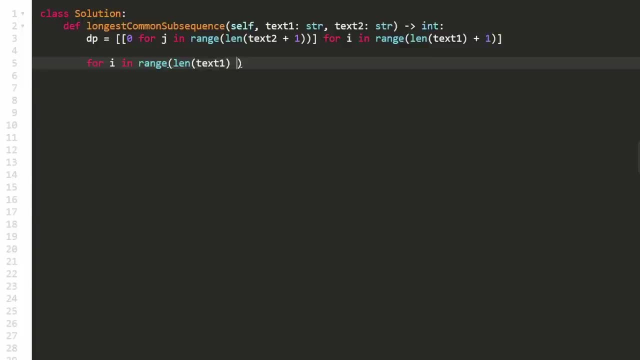 in reverse order. So in Python you can do it like this, And basically what I'm doing is starting at the bottom right of the matrix and then working our way up. So this is how you do it in Python: negative one, negative one, And let's do the same thing for text two, And so. 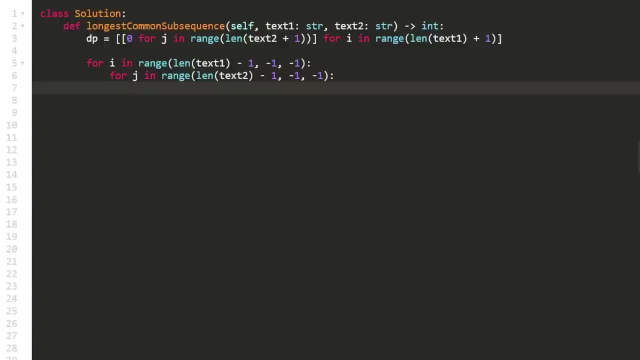 remember. so we're going through every cell in our 2d grid And remember there were two conditions. One condition is if the characters in both strings match each other. So if text one of I matches text two at position j, if they match each other, we're going to do. 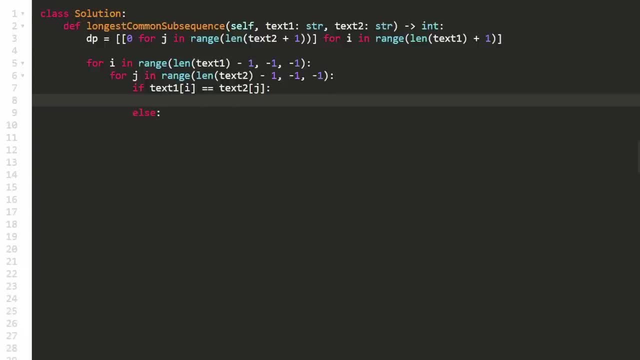 something, And if they don't match each other, we're going to do something different. So, remember, if they do match each other, then what we can say is, at this position, dp of i, j, because, remember, we're trying to fill in every single cell- what we can do is then just simply take one plus the. 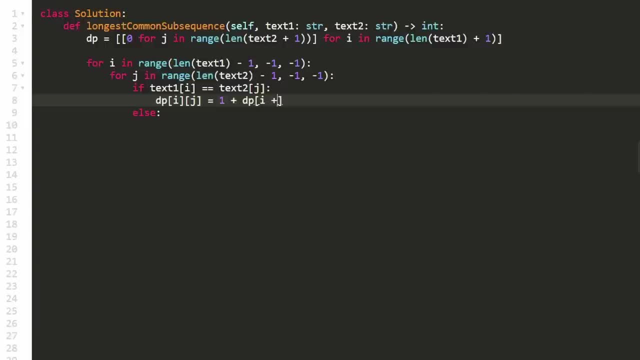 diagonal. how do we find the diagonal? Well, we can say well, we can say well, we can say well, i plus one and j plus one, right, that gives us the diagonal, And remember, we're adding one to it. 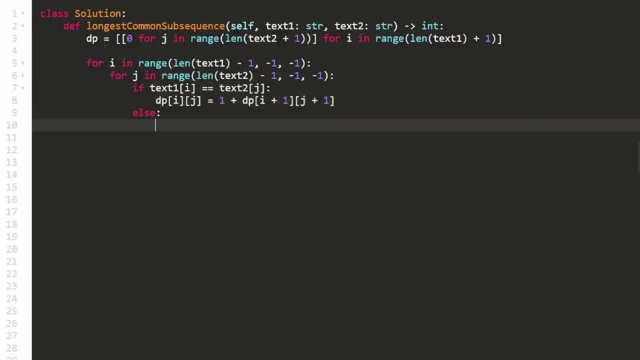 because these characters match, that means we add a one, And if they don't match, that's the else case, right? So we're doing something different here. we're going to put a different value for dp of i- j And in this case, what we're doing was we're finding the maximum of two values. what are?